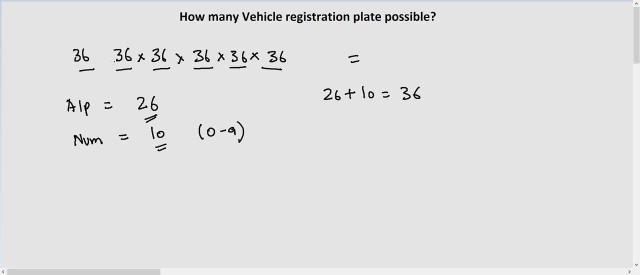 multiply all of these and that way we have 36 is to power 6 and that's the answer, right. so this is how many ways you can have a vital registration plate if you are using the alphabet, all of the alphabet and all of the numbers which 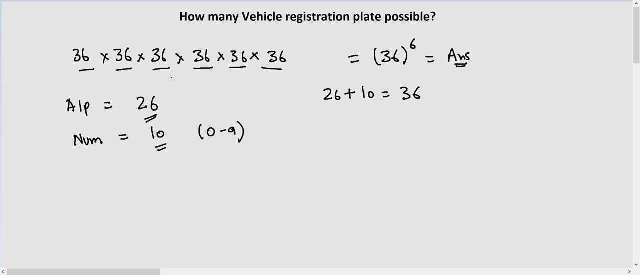 can go anywhere on the plate. now, in certain cases, we can have a restriction where the first two spaces has to be alphabet and the rest of the spaces have to be numbers. so this has to be numbers. so how will we calculate the possibility in this case? so that way, now, because we are choosing alphabet, we have 26. 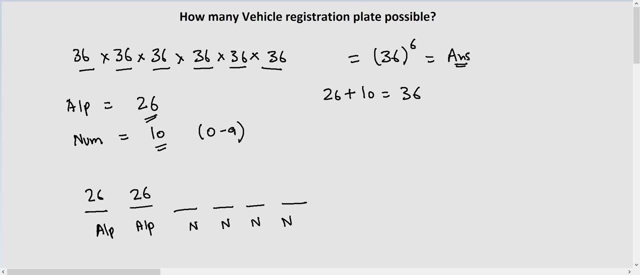 possibilities for the first two spaces. first one, 26 possibility for the second one and 10, 10, 10 and 10 for the other ones. now we multiply these and that will give us the answer. so the answer will be equal to 26 and 10 for. so that is the answer. now, if we say that we need a plate, 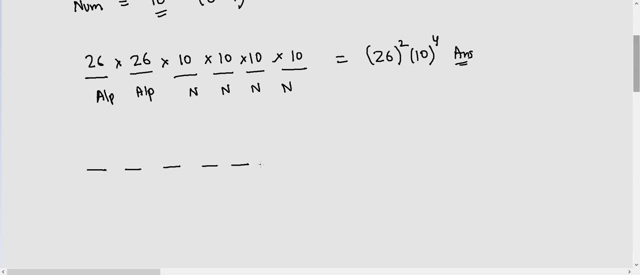 where the number should not be repeated. number or the alphabet should not be repeated. so now, in that case, it will be the similar scenario we saw for the people being arranged on the chairs, because the people cannot sit simultaneously at two different chairs. same way now, because we are saying the number cannot be repeated. 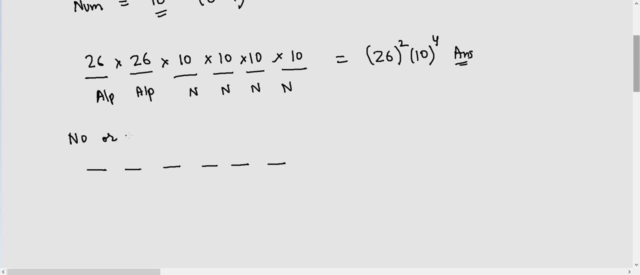 so number or alphabet can not be repeated now. the problem will completely change. so in this case, now for the first space we will have a number, and then we will have a number, and then we will have a number, and then we will do a field experiment in this course. but the